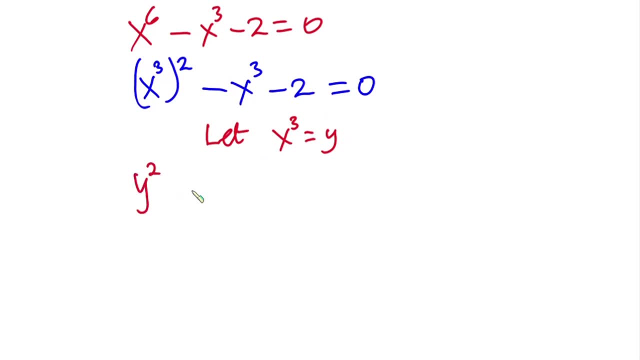 there. so we have y to the second power. minus y, minus two is equal to zero. all right, so from here i'll look for two values that when i multiply i'm gonna get negative two, but when i sum them up i'll be getting negative one, and the numbers are negative two and then one. okay, so i'll rewrite. 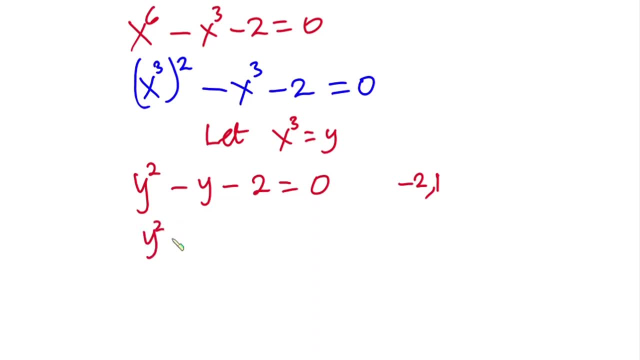 this equation as y to the second power plus y minus 2y minus 2 is equal to 0.. all right, so from here we have y here and then y here, so i can take y comma. so we have y plus 1. then from here we have. 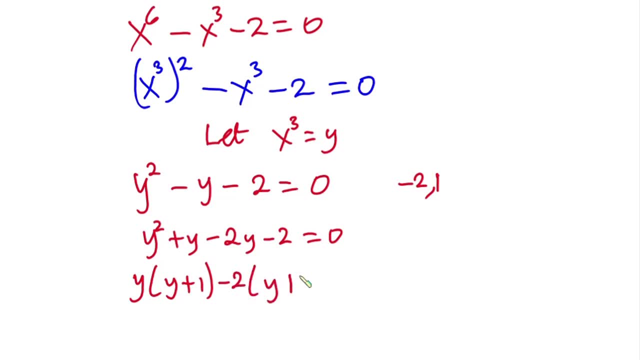 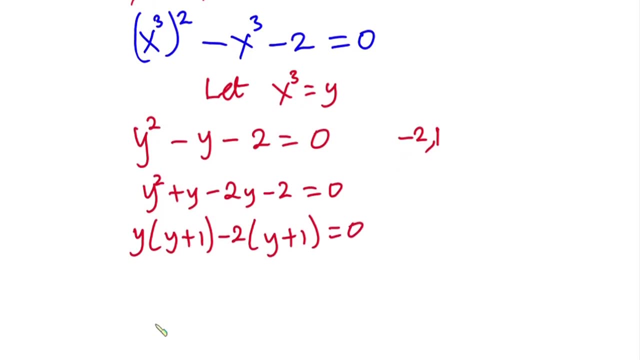 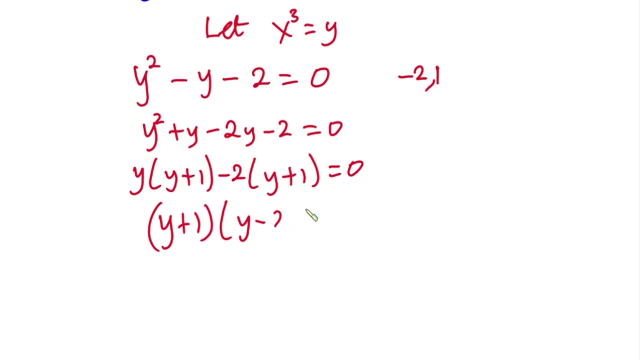 negative 2 into y plus 1, and this is equal to 0. okay, so from here we have y plus 1, then y minus 2 is equal to 0. all right, so from here we can say that y plus 1 is equal to 0 or y minus 2 is equal to 0.. so now let's make y the subject from. 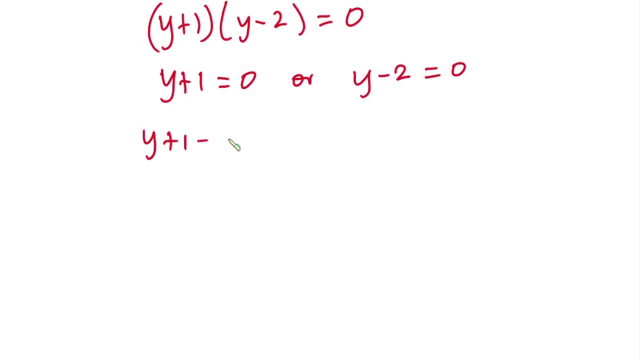 this equation. so we have y plus 1 minus 1 is equal to minus 1.. so this one will cancel this. now we have y equals negative 1. okay, then let's come to this side. so from here we have y minus 2 plus 2 is. 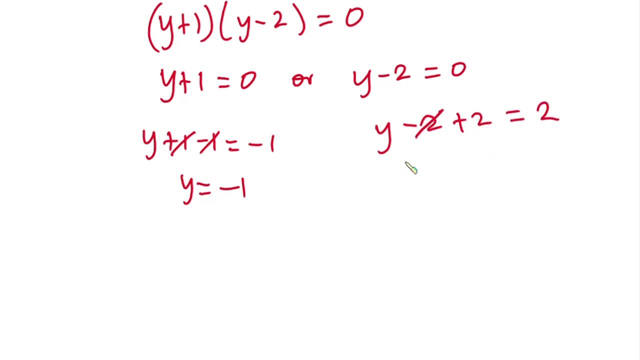 equal to 2.. so that this one will cancel this. now we have y equals 2.. but don't forget that we said x to the third power is equal to y, so when y is equal to negative 1, we have x to the third power equals negative 1. okay, equating. 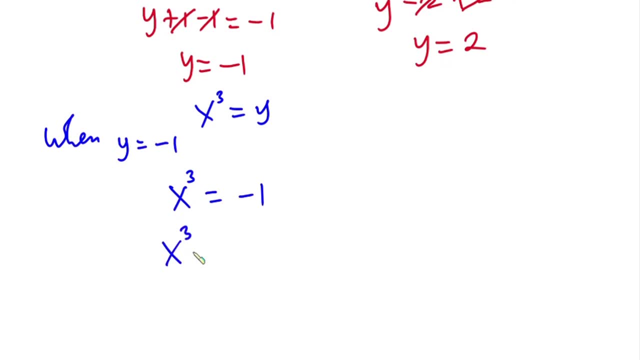 everything to 0. we have x to the third. power plus 1 is equal to 0 and don't forget, we have 3 over here, but you can choose not to write now. this whole thing is the same as x plus 1 into x to the. 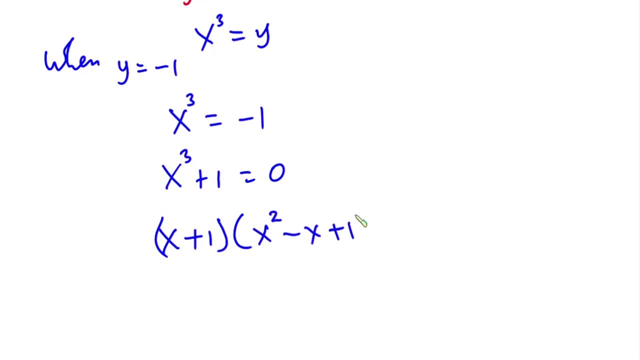 second power minus x plus 1 is equal to 0.. so we can say that x plus 1 is equal to 0, or x to the second power minus x plus 1 is equal to 0. all right, so from here let's make x the. 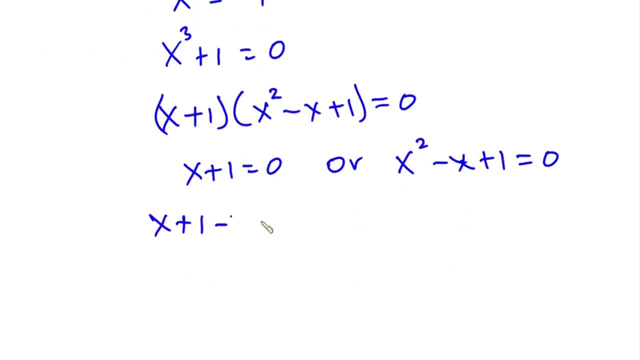 subject. so we have x plus 1 minus 1 is equal to negative 1.. so this one will cancel this. now we have x equals negative 1.. so this side we have x squared minus x plus 1 is equal to 0.. this is a. 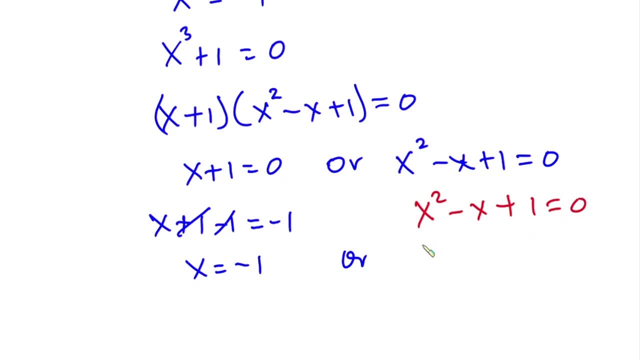 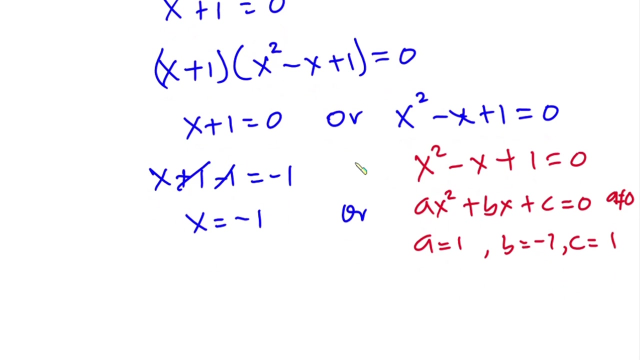 quadratic equation. so when we compare this one to the general quadratic equation, which is: ax squared plus bx plus c equals 0, where a is never equal to 0, we have a to be 1, b to be negative, 1, then c to be 1, all right. so now putting this into the general quadratic equation formula, which is: 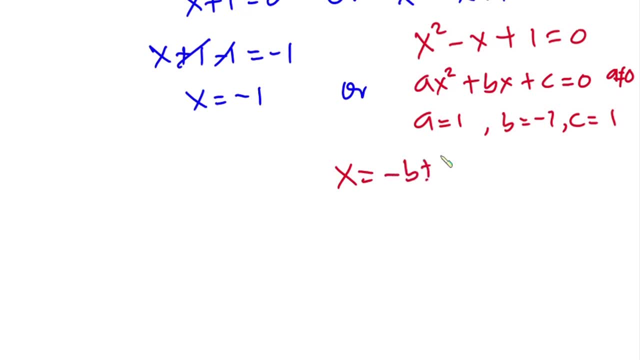 x equals minus b, plus or minus square root of b, squared minus 4 ac all over 2a. this gives us x equals 1 plus or minus square root of 3i all over 2.. so this implies we have x equals 1 plus square root of 3i over 2, and then x equals x equals 1 minus square root of 3i over 2. 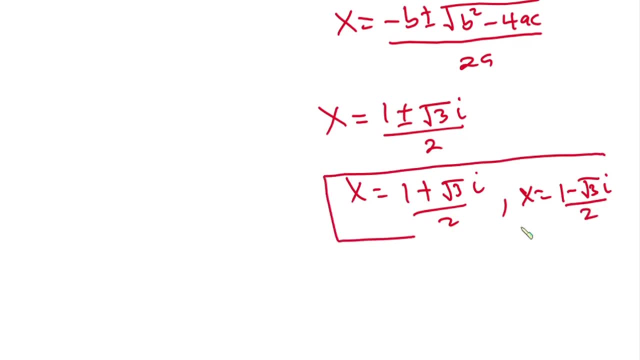 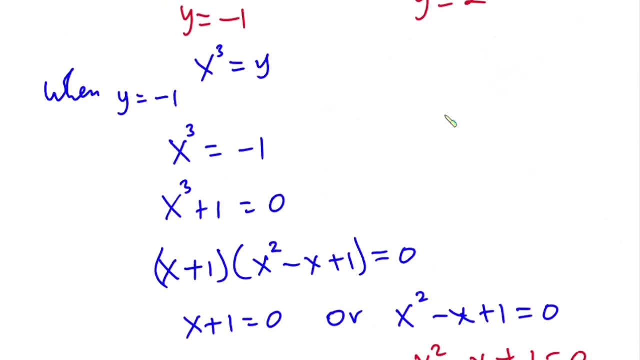 the reason why i didn't work this one out is because it is complex and we are not considering complex solution. okay, so now let's move on to when x equals 2. so what is the value of x when y equals 2? so when y is equal to 2, we have x. to the third power: 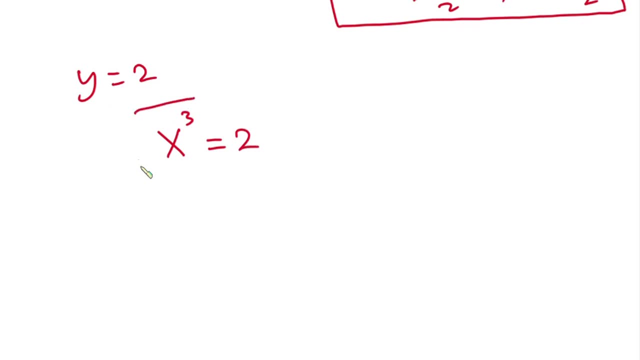 equals to 2. okay, so now, taking the cube root on both sides, we have this one, we take this now. we have: x equals the cube root of 2, and this is also the same as 2 to the power, one third. so this implies that x is equal to negative 1 or x equals 2 to the power. 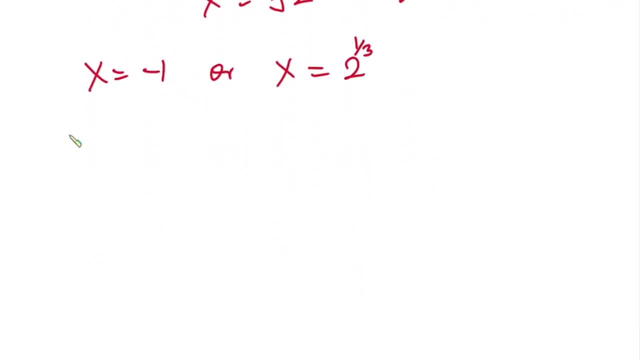 one third. now let's check and see. the equation is: x to the sixth power minus x to the third power minus 2 is equal to 0.. so let's see: when x is negative 1, we have negative 1 to the sixth power minus negative 1 to the third power minus 2 equals 0.. you can see that we have, even as the power over. 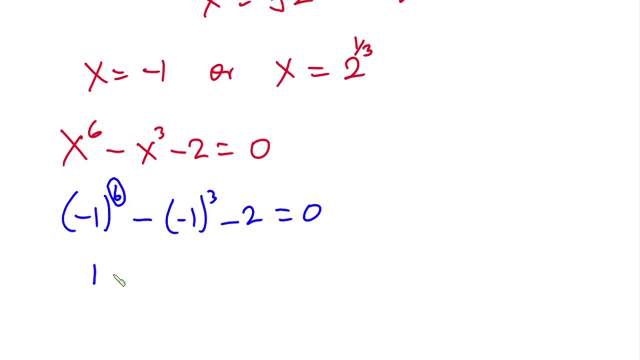 here. so this one becomes positive, 1, then minus, then this side. it is odd, so definitely this is negative. so we have negative 1 over here, then minus 2.. so we have negative 1 over here, then minus 2.. and this should be equal to 0. okay, so here we have negative. negative. it will be 1 plus 1, which? 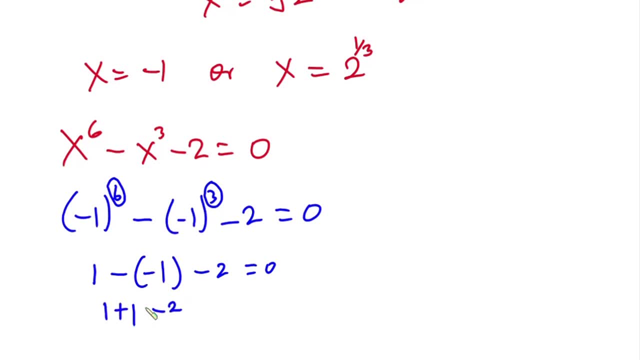 is positive, then minus this 2, then minus this 2, and this is equal to this, should be 0. okay, so we have 2 minus 2 should be equal to 0. so we have 2 minus 2 is definitely 0. okay, so we can say that. 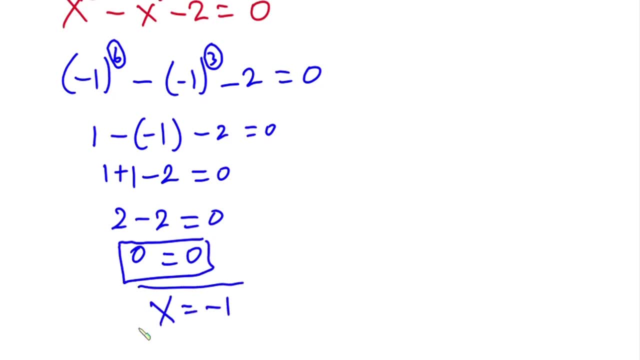 x equals 2.. because negative 1 is a real solution. okay, now let's test and see: when x is equal to 2 to the power one third, so when x is 2 to the power one third, we have 2 to the power one third. 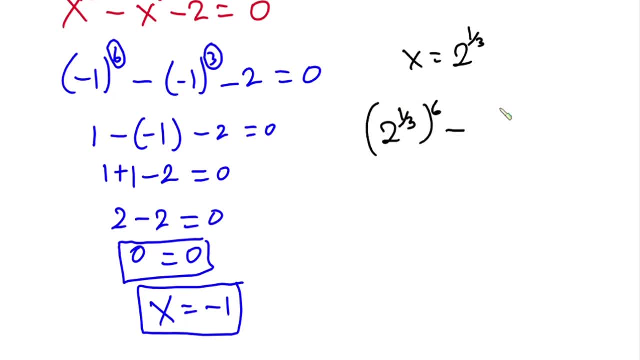 or to the power six minus two to the power one third. one third to the third power minus two. it should be equal to zero. so from here we have two to the power two. okay, then minus two, because this one will cancel this. okay, then minus two is equal to. 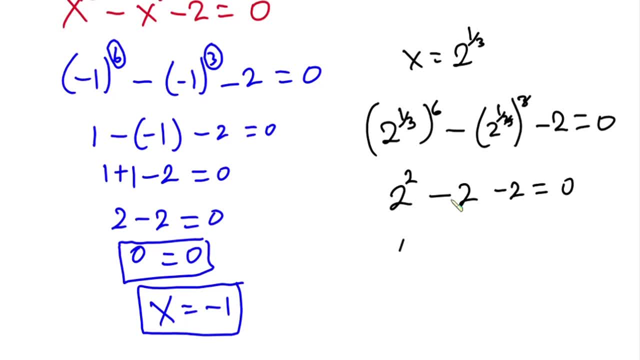 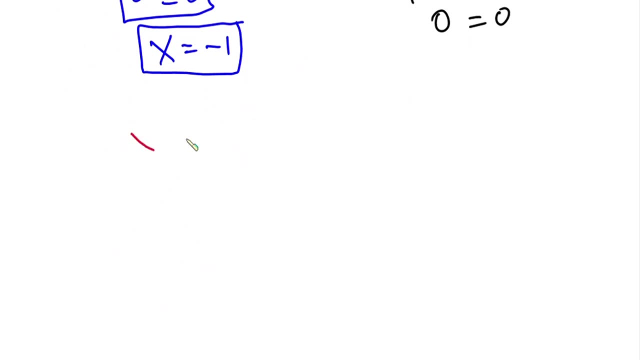 zero. so here we have: two squared is four, then two minus two is nothing but four, and this should be equal to zero. and of course, four minus four is equal to zero. so we can say that the final answer to this problem is: x is equal to negative one and then two to the power.